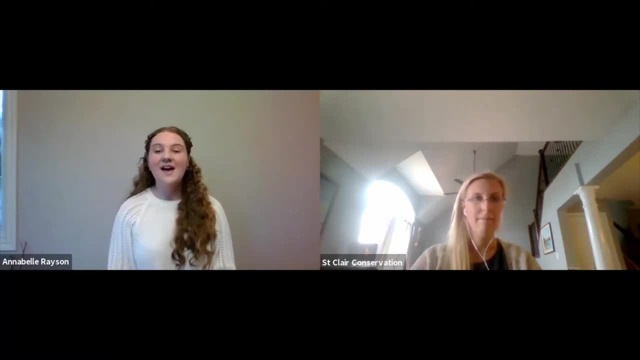 algae, Chlorella and Selenostrum in four different concentrations: 25%, 50%, 75% and 50%. My hypothesis was that the Daphnia magna would be the most effective independently, as they are the largest sized filter feeder in the experiment. The combinations containing amphipods: 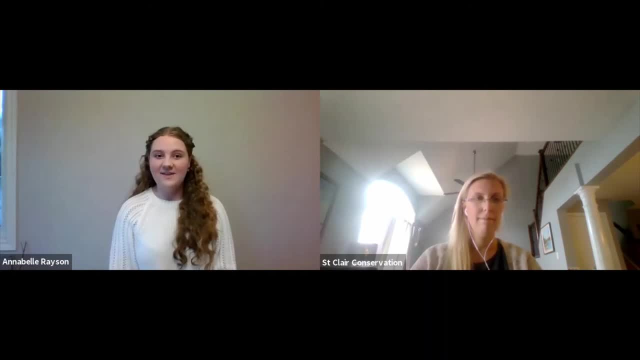 should be the least effective, as amphipods are omnivores and will likely consume the other species of zooplankton they are combined with first. The combinations containing Daphnia magna again, should be the most effective due to its larger size, and the Selenostrum should. 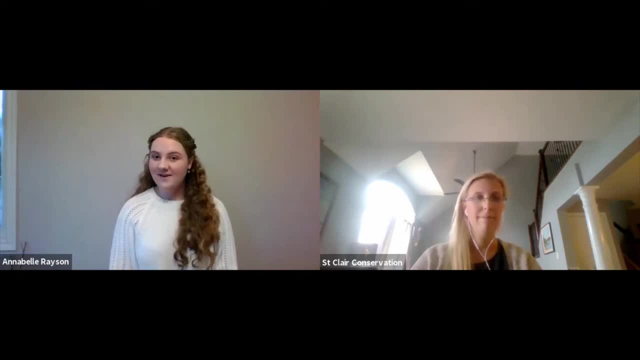 be the algae with the most decreases, as it's a microalgae and easier for the filter feeders to consume. For my procedure, I took 264 little plastic cups and I ensured that each cup had 12mL of liquid with the different algae concentrations and that each cup except for my controls. 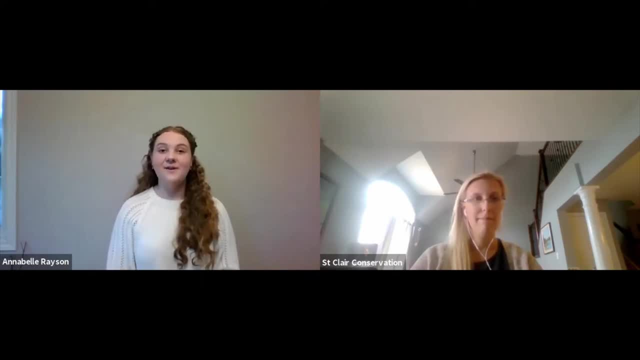 had precisely 6 zooplankton in them. I then let this sit for a two week period and once that was up, using a hemocytometer in my microscope I counted the algae cells in each of the samples, and then I used excel spreadsheets to make calculations. 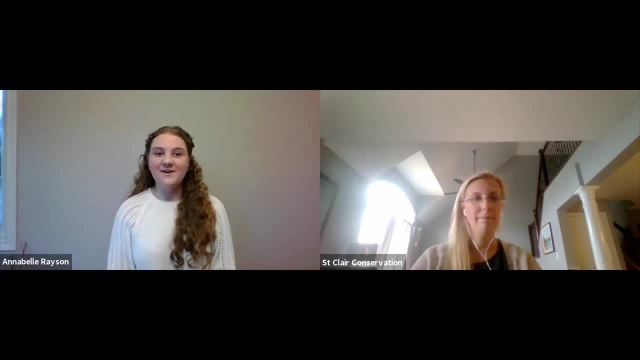 I discovered that the Daphnia magna was the most effective species of freshwater zooplankton to biomanipulate. As when counting the algae, I counted the algae cells in each of the samples and then I used excel spreadsheets to make calculations. I discovered that the Daphnia magna was the most effective species of freshwater zooplankton to biomanipulate. I made a test result and when I tested on Chlorella algae, it resulted in an average algae decrease of 89%. and when tested on Selenostrum algae, Daphnia magna, resulted in an average algae: decrease of 98%. …And by discovering the best species of freshwater zooplankton, Daphnia magna, to biomanipulate, to increase its presence, to prevent and treat harmful algae blooms, the future of algae bloom treatment and prevention is much clearer. 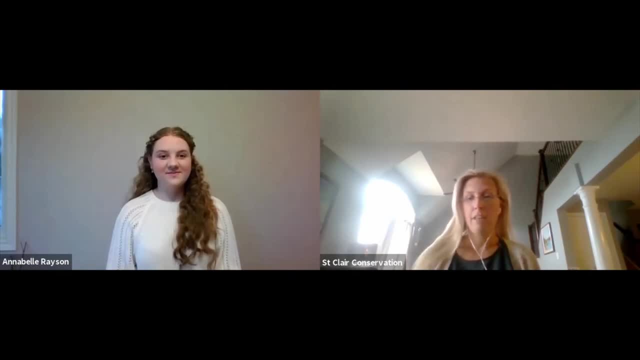 Wow, That was awesome. I love the diversity in the number of species you chose, the different concentrations that you looked at and, I think, a really well thought out, in-depth research project. especially for someone in grade 10, that's phenomenal. So can you tell us how like was this? 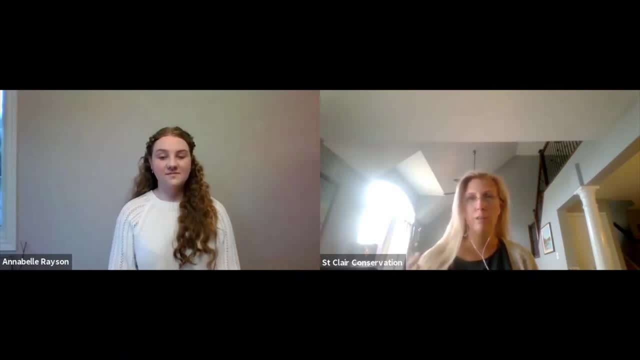 a research project you needed to do for high school or for a bigger science fair. what was this connected to? So this was something I did independently for the past. this is my sixth year- I've participated in the Lampin County Science Fair, the local science fair in Sarnia, and I've 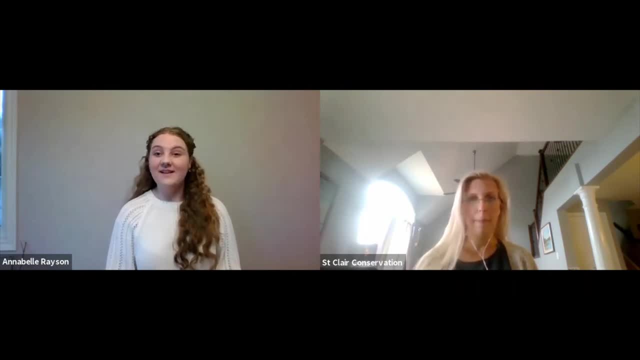 always been. my projects have always been on environmental sustainability and, living in South Western Ontario and being surrounded by the Great Lakes and our beautiful freshwater ecosystems, I've always developed a passion for them, and when I learned about harmful algae blooms, I was kind of more interested in looking at the causes of them and ways to prevent and treat them. and so for my 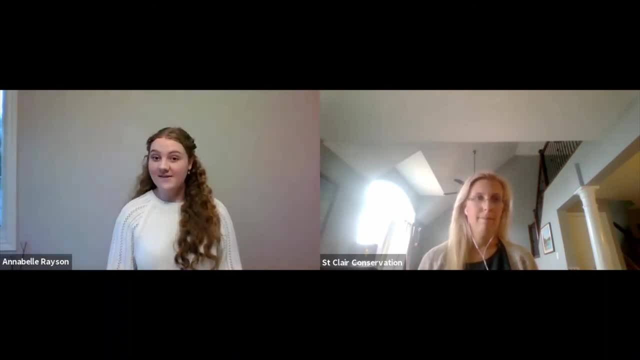 project this year. I chose to look at different ways to decrease and prevent harmful algae blooms and I chose to focus my project on the process of biomanipulation and using zooplankton and, as a matter of fact, I've actually placed best and fair at the Lampin County Science Fair and I'll be progressing on to Youth. 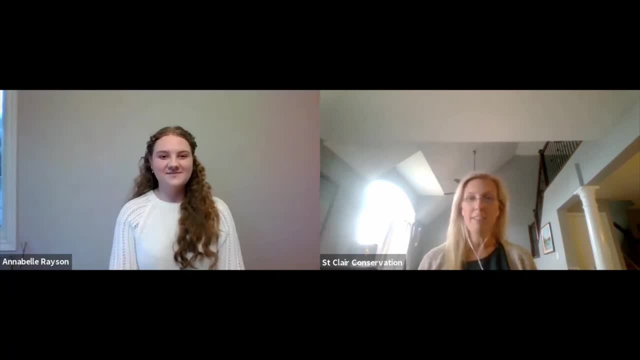 Science Canada's Canada-wide science fair in May. That is incredible, and what does that entail? Well, traditionally it's virtual this year, but it's usually a week-long event at a different host city in Canada, with competing against the 500 best and brightest science fairs. 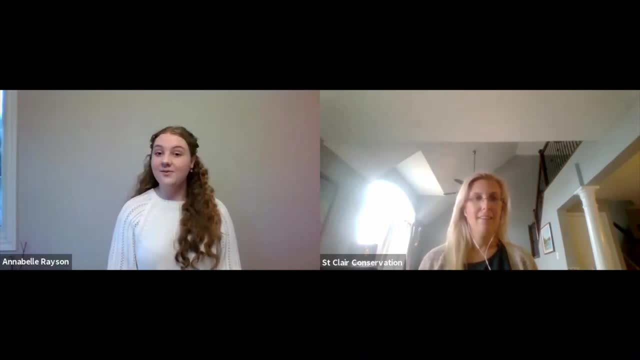 and so this year, since it's virtual, it's themed in Ottawa, and so we'll have virtual calls with judges, similar to what we're doing today, and we get to create and produce little virtual boards, and there'll also be different virtual tours and events to keep morale high. 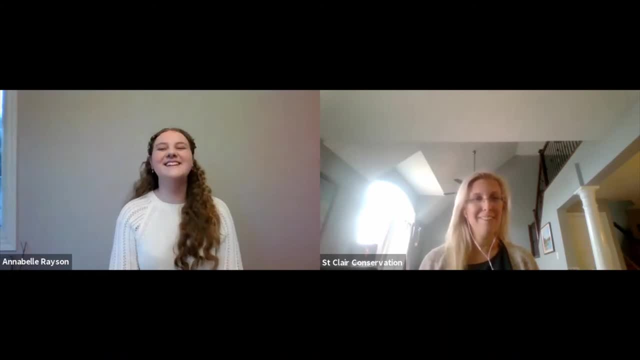 Awesome. this is kind of like a little warm-up then for you. that's awesome. Now, who did you work with It sounds like this is quite a big project. I think earlier you and I were talking about your living room and your kitchen. Can you tell us a bit more about who you worked? 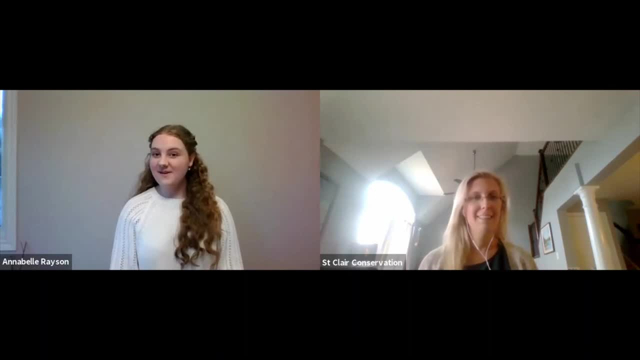 with and how you set up the project. So I spent about six months researching this concept on my own and through. I did my experiments in my living room, my kitchen, and my family's been incredibly supportive and helpful with this and whenever I've come up with little hiccups or guidance questions. 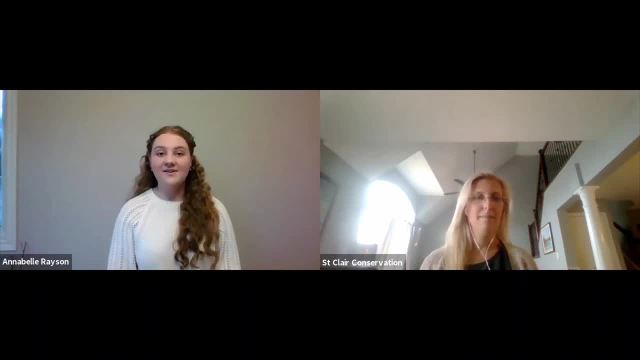 I've actually some of my algae zooplankton were provided to me from Clay Ferguson and his team at Paulwood Tech in town, Which is a local biology lab, and then I've also worked with Marian Racine from Environment and Climate Change Canada. She's helped me when I've come up with hiccups on how to calculate and 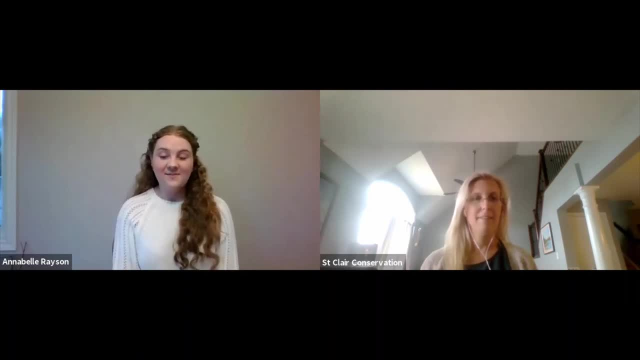 figure out different ways around my project and to expand my research. I've also worked with Curtis Tamming at Lampden College. He's provided me with calculation assistance and lent me the hemocytometer. and Diane- Mrs Diane Yerkewich, my curling coach and teacher at St Pat's. 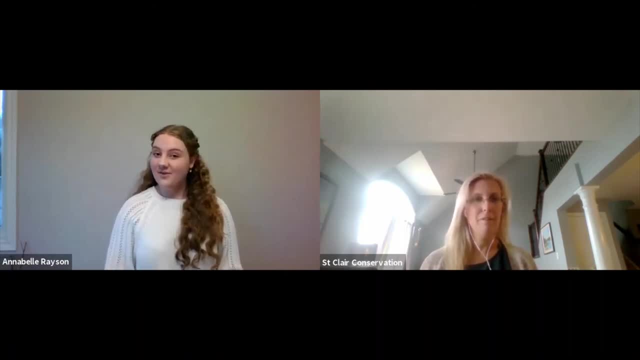 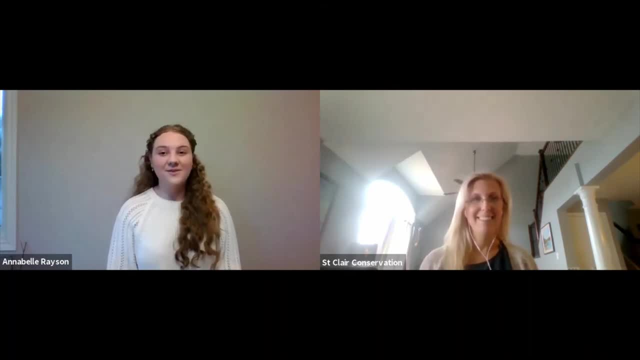